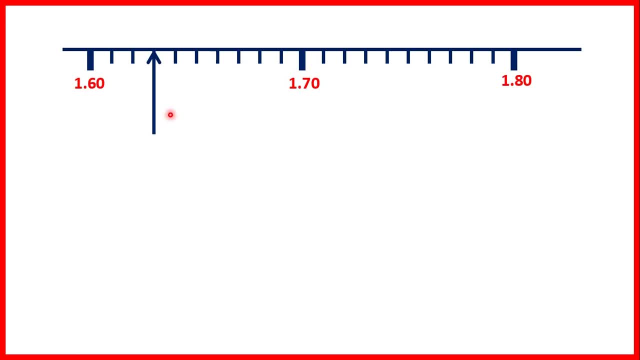 So then, if we need to find a specific value, it's easier for us to work out. This line is pointing to 1.63, because we're three lines after 1.6.. Here we have 1.68, then 1.74, because we're four lines after 1.7.. And here we have 1.6, 1.7 and 1.8.. Here we have 1.64 because we're four lines after 1.7.. And here we have 1.68 because we're four lines after 1.7.. 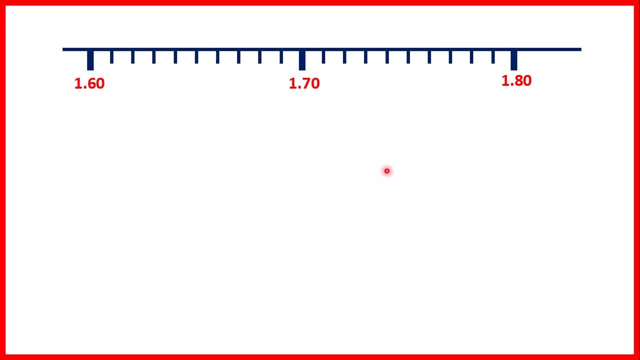 have 1.77.. Now this number line is slightly different. We have 0 and our tenths and 1 as our labelled values. Again, we can put zeros on the end and if we've got a whole number, we can write .00 on the end. So we can do that with 0 and 1.. So what number is the arrow? 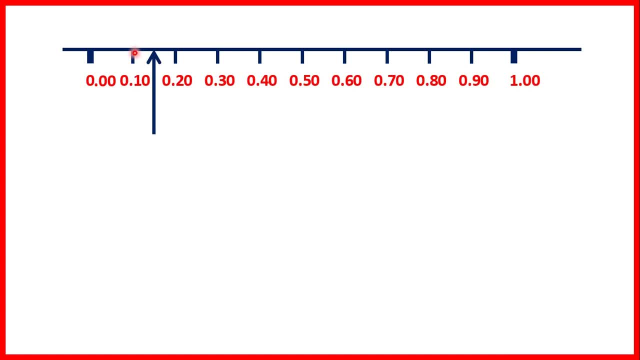 pointing to. Well, between 0.1 and 0.2, we have 0.15.. That's right in the middle and it makes sense if you think that 15 is right in the middle of 10 and 20.. So where is the arrow? 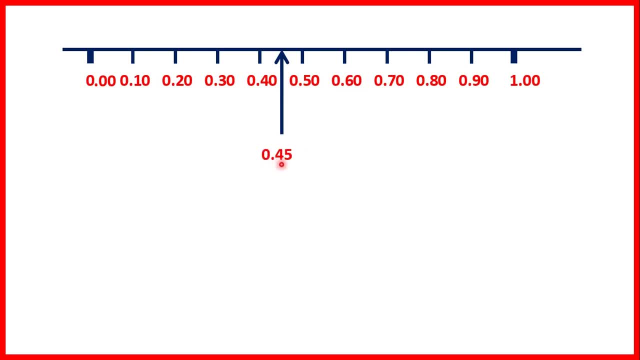 pointing to now? Well, this is 0.45.. That's right in the middle of 0.4 and 0.5.. So what number is the arrow pointing to? Well, between 0.1 and 0.2, we have 0.15. That's. 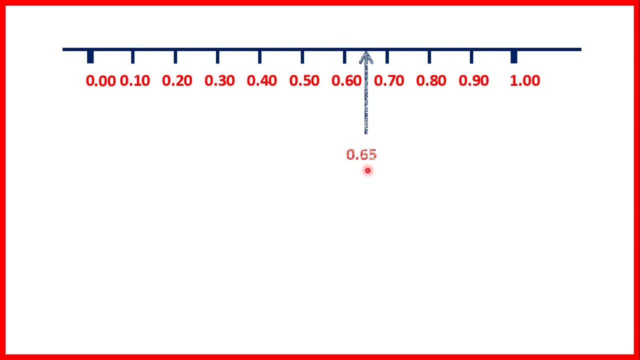 0.15.. That's right in the middle of 0.4 and 0.5.. Now we have 0.65, and here the arrow is pointing right in the middle of 0.9 and 1,. so that's. 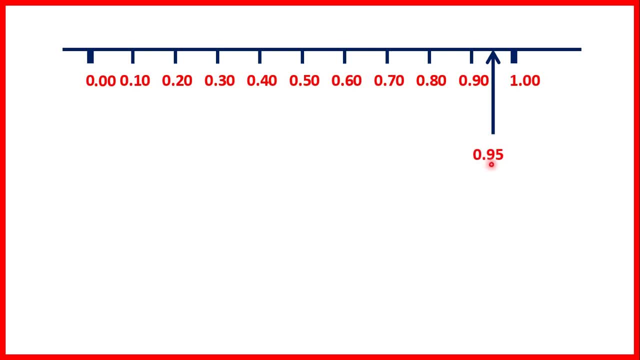 0.95, and that makes sense, because 95 is right in the middle of 90 and 100.. Now for this number line, we have 0,, 1, and 2, so we have whole numbers labelled, and this 0.5 tells us that each of these lines must be 1 tenth, because 0.5 is 5 lines after. 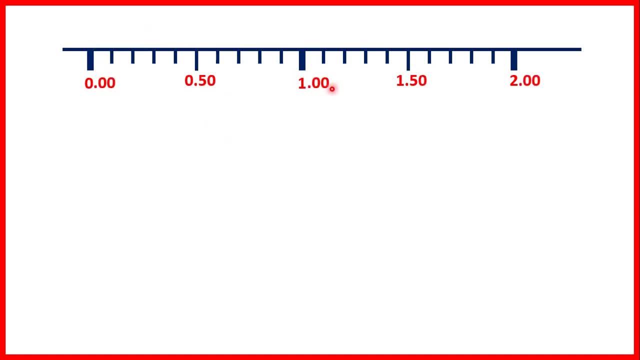 0.. Again, we can put zeros on the end of decimals without changing them, and if we have whole numbers, we can always write 0.00 on the end of decimals, Because that will help us work out the values that we need. 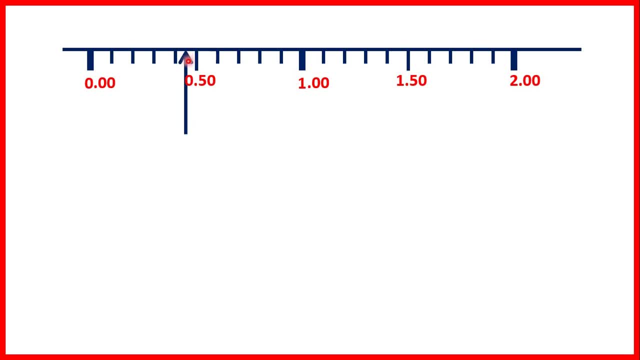 So which number is the arrow pointing to here? That's 0.45, because, remember, each of these lines is 1 tenth, and so this line here is 0.4,. we have 0.5 labelled, so right in the middle we have 0.45.. 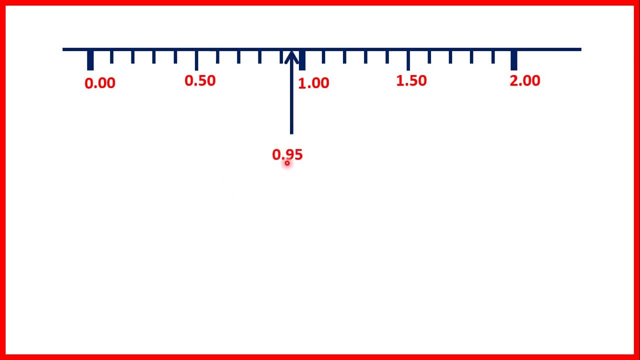 Here we have 0.95.. That's right in the middle of 0.9 and 1 whole. What number is the arrow pointing to now? Well, that's 1.35, because this line here is 1.3, the line after the arrow is 1.4, and 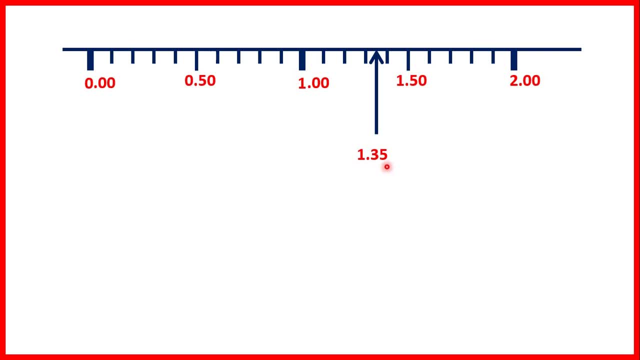 the arrow is right in the middle, so that's 1.35.. And where is the arrow pointing to now? Well, we have 0 and 0.5.. That's 0 and 0.1.. So right in the middle, we have 0.05.. 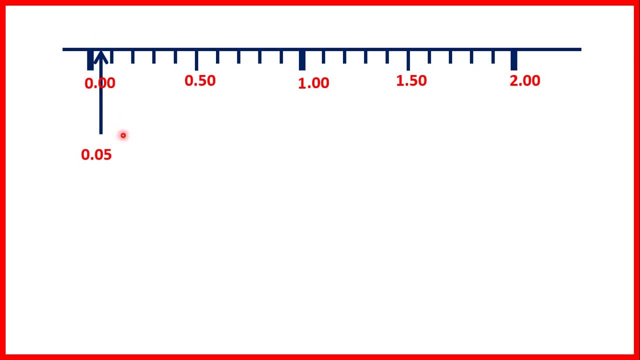 That's right in the middle of 0 and 0.1, because that's equivalent to five hundredths, And if we double five hundredths we have 10 hundredths and that would be 1 tenth. So now onto our last number line. again, it's easier to find values if we write 0s. 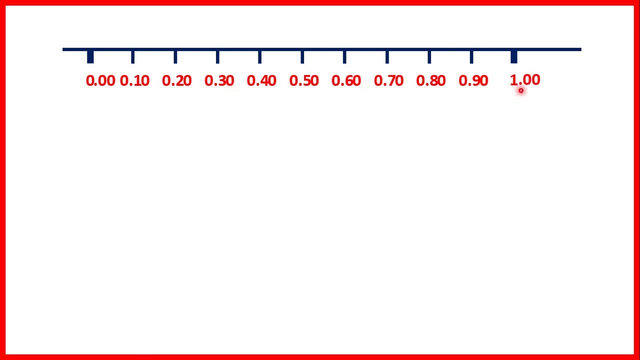 on the end of our decimals, And that's because we have 0 and 0.1.. And if we have whole numbers, we can always write 0.00 on the end, so that we have two digits after the decimal point, just like we have with all of our other values. 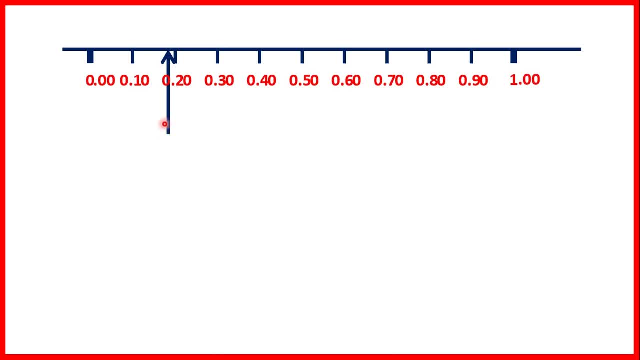 So where is the arrow pointing to here? Well, we can see that the arrow is now not right. in the middle, The arrow is closer to 0.2 than 0.1.. So I would estimate that the arrow is pointing to 0.18.. 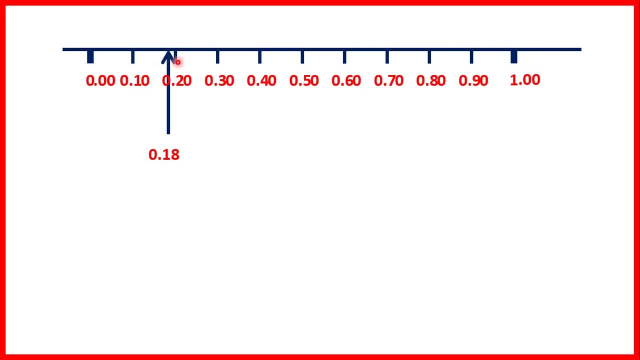 Or perhaps 0.17 or 0.19, but definitely more than 0.15.. So where is the arrow now? It's closer to 0.4 than 0.5.. So I would estimate it's at 0.43 or perhaps 0.42.. 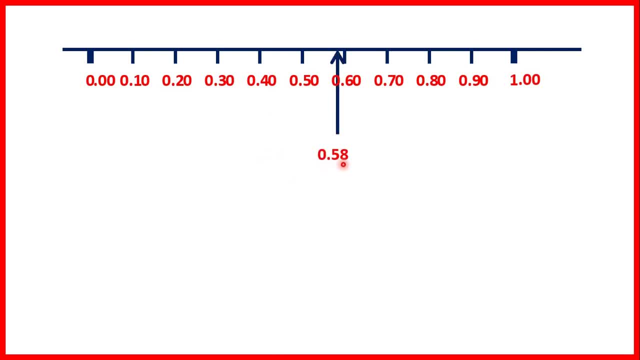 Here the arrow is pointing to 0.58, because it's closer to 0.1. So I would estimate that the arrow is now closer to 0.4 than 0.5. So I would estimate it's at 0.43 or perhaps 0.42.. 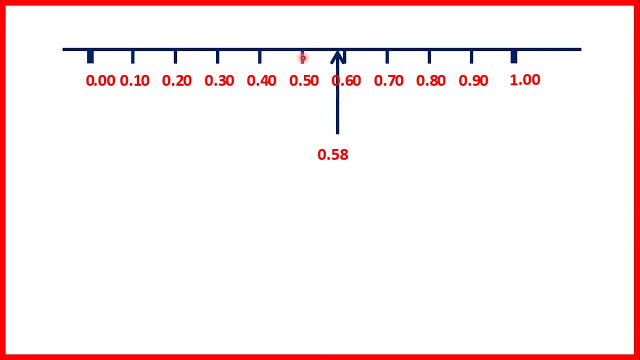 So I would estimate it's at 0.43 or perhaps 0.42.. And finally, here we can see, the arrow is almost in the middle of 0.9 and 1, but perhaps just slightly closer to 1.. So I would estimate 0.96.. 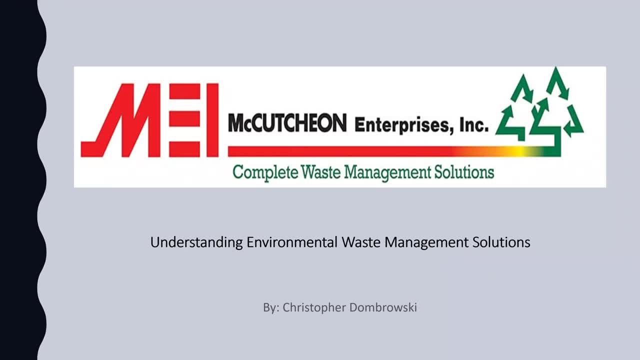 Hi, my name is Christopher Dombroski. Over the summer I had the opportunity to intern with McCutcheon Enterprise Incorporated doing environmental waste management and chemical analysis. So here's a little bit about me. I am from Pittsburgh, Pennsylvania, and I'm a junior. 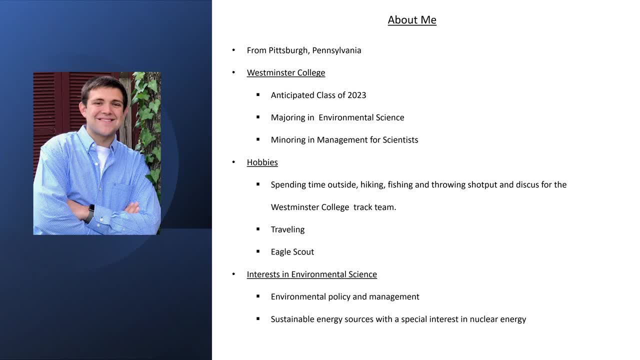 at Westminster College. I am majoring in environmental science and minoring in management with scientists. My hobbies include spending time outside, hiking, fishing and throwing shot put and discus for the Westminster track team. I also enjoy traveling and I am the 200th Eagle. 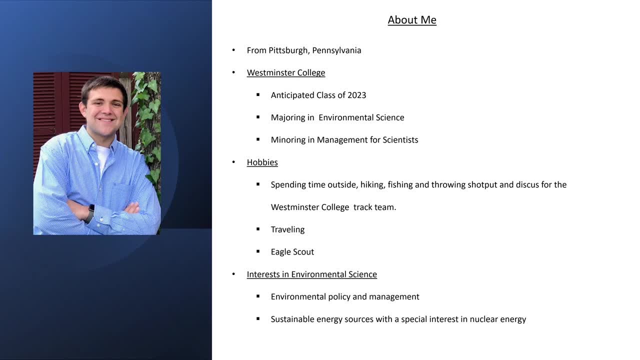 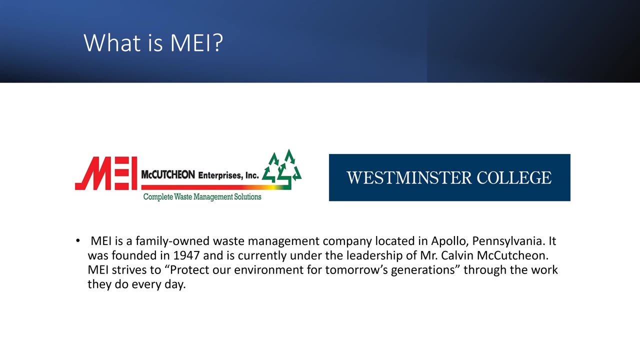 Scout of Boy Scout Troop 186.. My interests in environmental science consist of environmental policy and management, along with sustainable energy sources and a special interest in nuclear energy. So what is MEI? The company I interned with this summer was McCutcheon Enterprise. 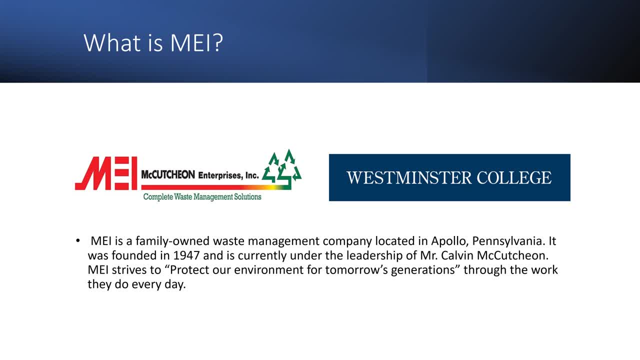 Incorporated. MEI is a family-owned waste management company located in Apollo, Pennsylvania. It is a family-owned waste management company located in Apollo, Pennsylvania. It is a family-owned waste management company located in Apollo Pennsylvania. It was founded in 1947, and is currently under the leadership of Mr Kelvin. 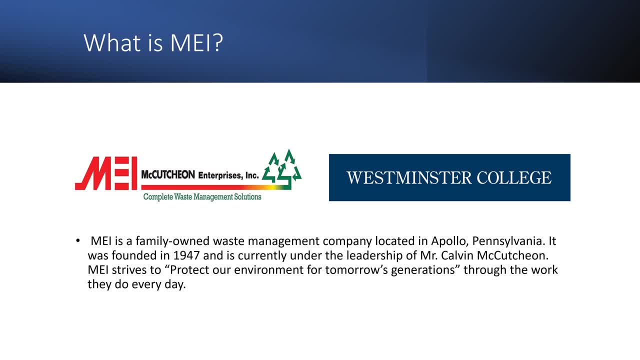 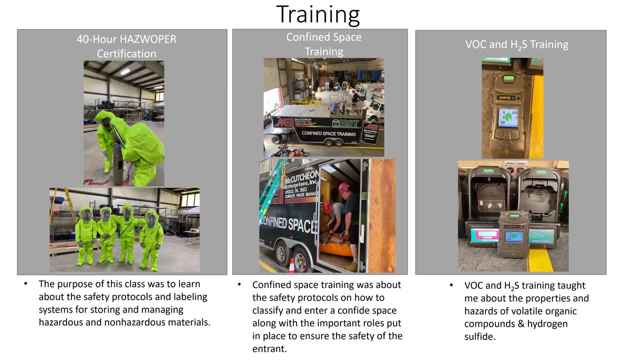 McCutcheon. MEI strives to protect our environment for tomorrow's generations through the work they do every day. Let me tell you about some of the training I received at MEI over the summer. Prior to working in the field, I was required to take several training courses. Each training 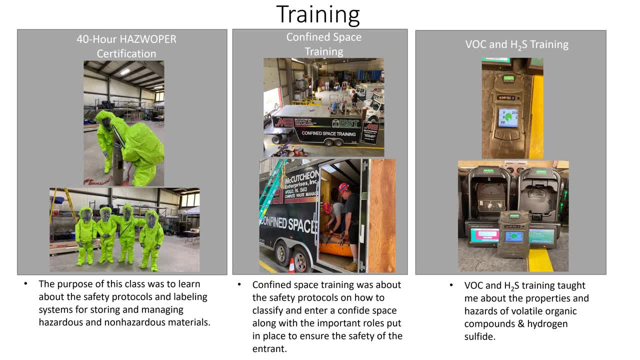 courses consisted of the 40-hour HAZWOPER certification, confined space training and research and development. I was also required to take several training courses. Each training course consisted of the 40-hour HAZWOPER certification, confined space training and research and development. I. training, confined space training and research and development. I was also required to take several training courses. Each training course consisted of the 40-hour HAZWOPER certification, confined space training. confined space training and research and development. I was also required to take several. training courses. Each training course consisted of the 40-hour HAZWOPER certification- confined space training, confined space training and research and development. I was also required to take several training courses. Each training course consisted of the 40-hour HAZWOPER certification- confined space.